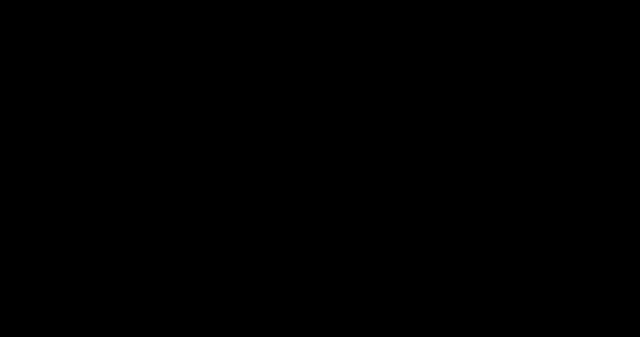 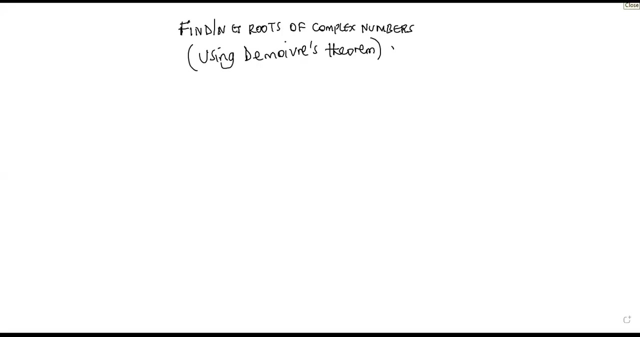 Well, in our previous video we looked at how we use De Mova's theorem to prove trigonometric identities, But in this video we are going to cover how we can find the roots of complex numbers using De Mova's theorem. This is somehow kind of yeah, but we shall get it very well. 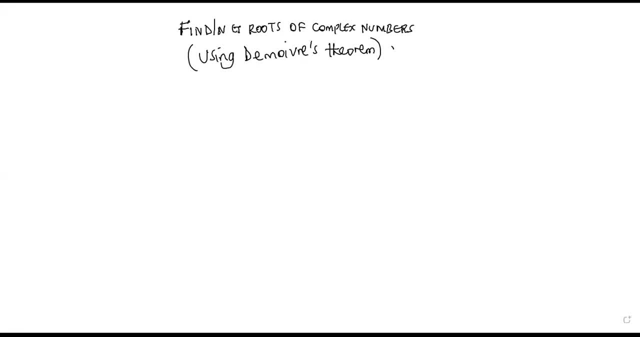 but we just need to pay maximum attention. And there are other methods. There is another method that we can use to find roots, but in case they say using De Mova's theorem or De Moiva's theorem, so you need to be knowing this approach also. So 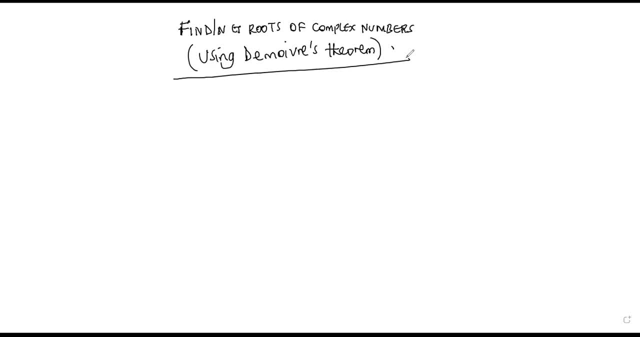 it's very easy. realistically, provided we know how to get modulus, provided we know how to get the argument, It is very, very, very easy, very, very, very easy for us. So now we're going to suppose, I'm supposing- 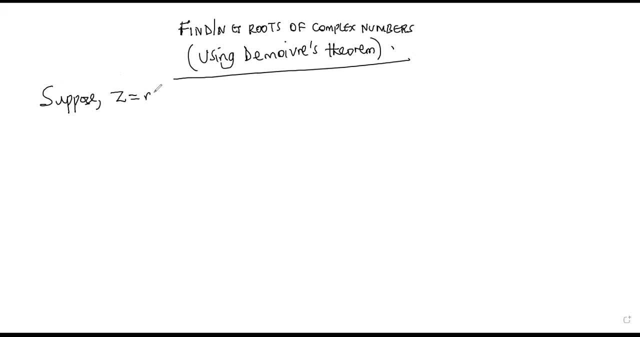 you know, z over r has always been in a polar form: r with theta plus i sine theta. That is our z. It means that z power n 0, equal to r power n cos n theta plus i sine n theta. All right. 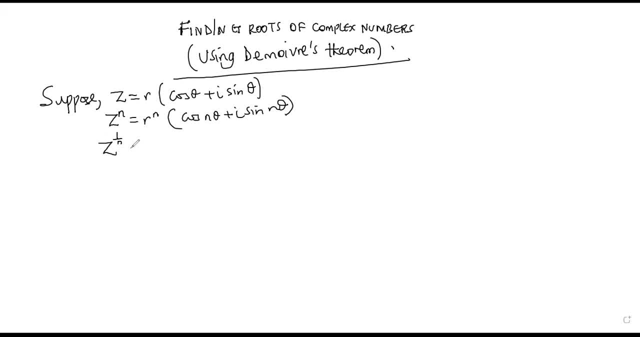 Knowing that if we have z power 1 over n, it's the same as r power 1 over n, cos 1 over n theta plus i sine 1 over n theta 0. So the general expression for finding roots of a complex number of complex numbers. 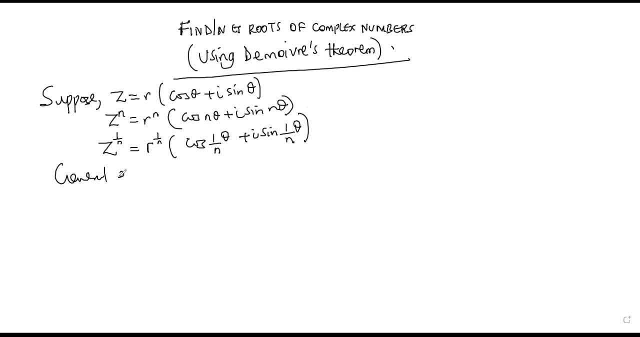 is given by- we call it general expression for finding roots of complex numbers- is given by: z is equal to r 0. 0.. into cos theta plus two pi k, then plus i, sine theta plus two pi k. right where k, k is given as zero, one, two a, t, c and theta is normally given in radians, you can always. 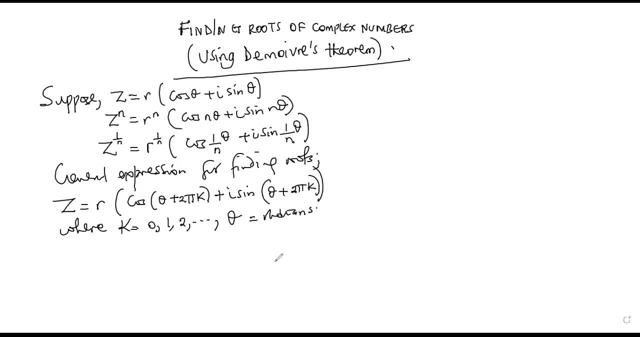 express our theta in radians. now, for any root, for any root of a complex number. uh, it would mean that z power n would be equal to z power n would be equal to r power n. cos n theta plus two pi k right then, plus i sine um. 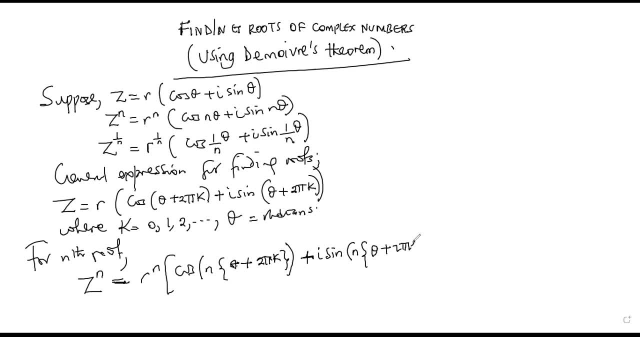 n. theta plus two pi k, right, uh, meaning that for one over nth root, for one over nth root, it would mean that z power one over n be going to r power one over n. cos theta plus two pi k over n. plus i sine theta plus two pi k. 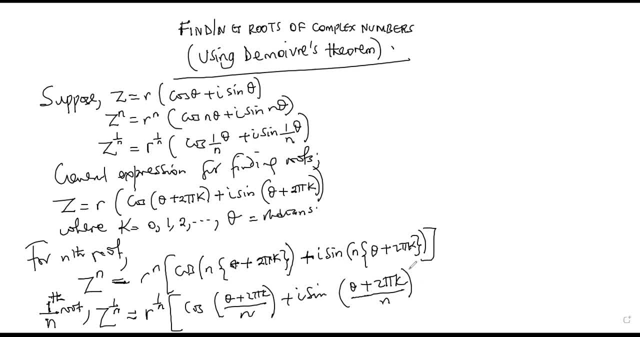 over n. we need to quote this formula for all the processes we are going for. that is how we get the any, the one over nth root of a complex number. okay, uh, so we are going to have some examples. um right, uh, we are going to have some examples. 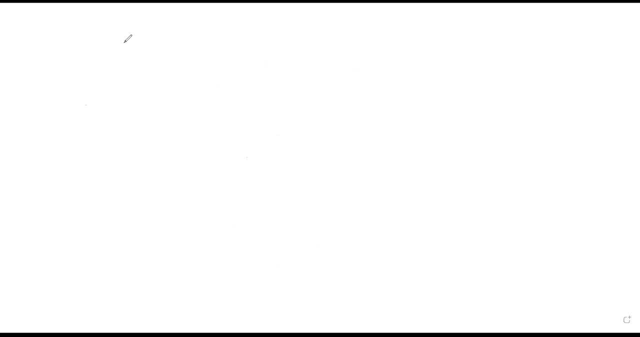 and uh. the examples are: use the movers theorem. use the movers theorem. find the square root of roman one, three plus four. i roman. two minus three minus four, i roman. three, five minus twelve, i. uh, i will do part one and um, i will do part one and. 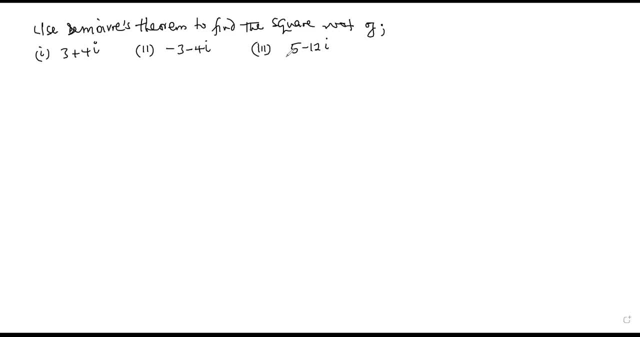 two, then expectedly you do, but three, then other examples will come on. uh, for this part we are having. for this part we are having this, but from our formula we need to get the magnitude of z, which will be the square root of 3 squared plus 4 squared. this is 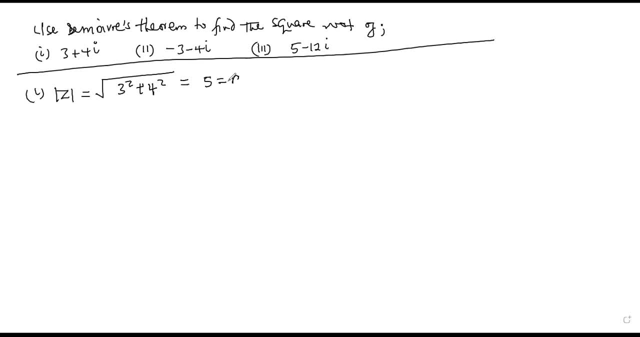 5, and this is the same as our R. So our R is five. okay, Our R is five. And the argument of Z, which is equal to theta, is the tan inverse of Y over X, which is four out of three, And this is: 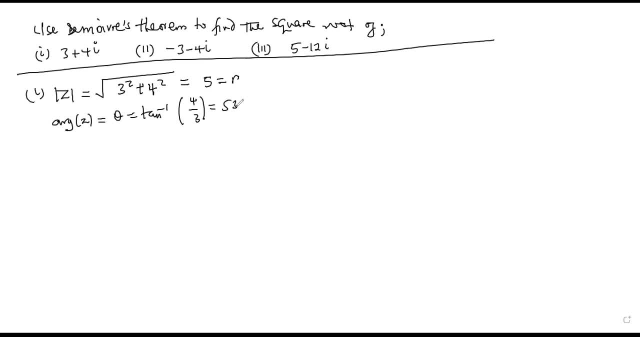 equal to 53.13.. If you put this in radians, okay, Okay, you can even draw to show where it would really lie. So here we have the imaginary and there we have the real. So we have four: three. So real is three, imaginary is four. So we have it, here It. 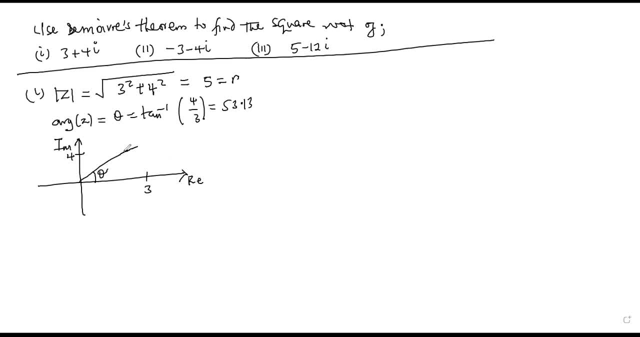 makes it with a positive x-axis. So this is our four and this is our five. So you can see that we have a positive x-axis and we have a positive x-axis. So we have a positive x-axis here in the second row. 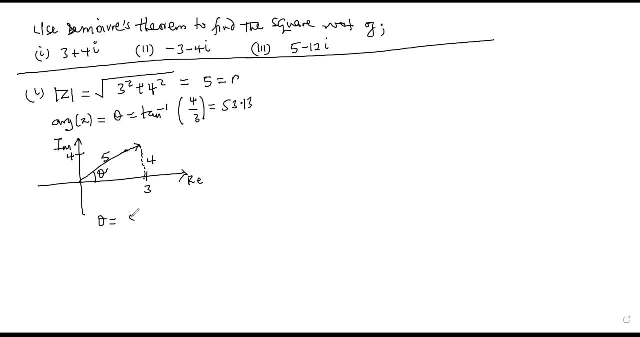 So it doesn't say that it lies in the first quadrant. It lies in the first quadrant And therefore theta is equal to 53.13, which is equal to when you put it in radians. I say you say 53.13 pi out of 180. And this will give you 0.295 pi. 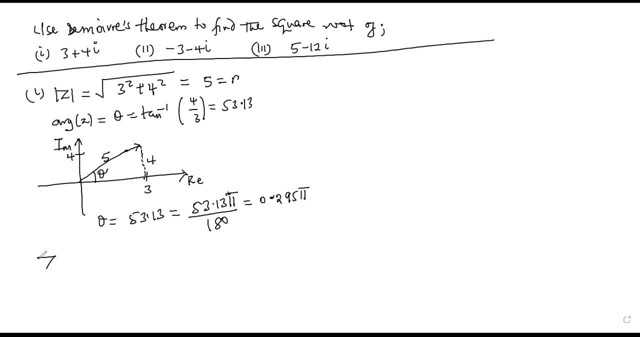 Okay now it means that our z would be equal to r. you check on the other forms, it would be r, which is 5, into cos theta, which is 0.295 pi plus 2 pi k plus i sine. 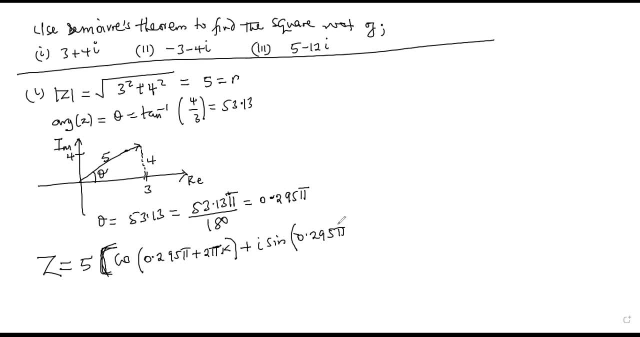 theta 0.295 pi plus 2 pi k, meaning that if we need the square root z power a half, we'll be calling it to 5 power a half into cos theta 0.295 pi plus 2 pi k over. 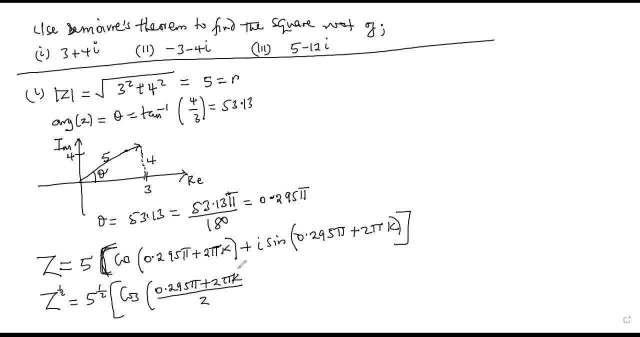 theta 2, any 2, then plus i sine 0.295 pi, plus 2 pi k over any which is 2.. Right now, having that, since we are looking for the square root, we shall that value. 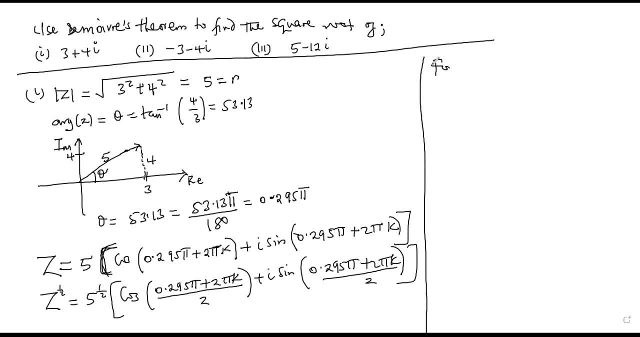 of k we shall be substituting. So for k is equal to 1, we begin with a 0.. For k is 0, we shall get z1.. So z1 will be equaling to 5 power a half into cos. k is 0, so the whole of this is: 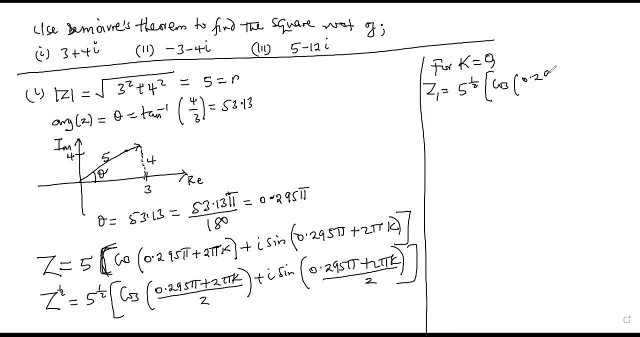 0,, so we shall have cos 0.295 pi over 2, plus i sine 0.295 pi out of 2.. Right, So z1 will be equaling to 5. power a half into cos k is 0,, so the whole of this is 0, so we shall have cos 0.295 pi over 2,, plus i sine 0.295 pi out of 2.. 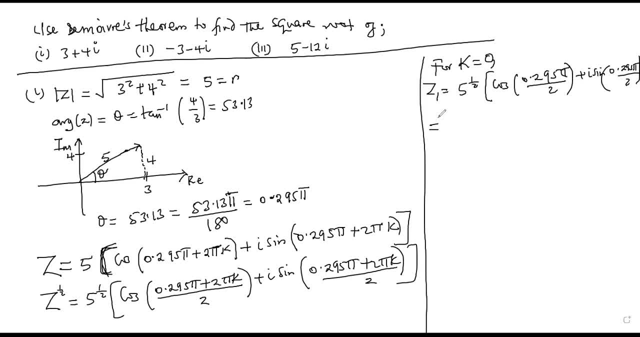 Right, So this is going to be. I'm putting on my calculator, I'm putting on my calculator. If you put on your calculator also, this is going to be equal to well, okay, so it's going to be equal to. this will reduce to two. 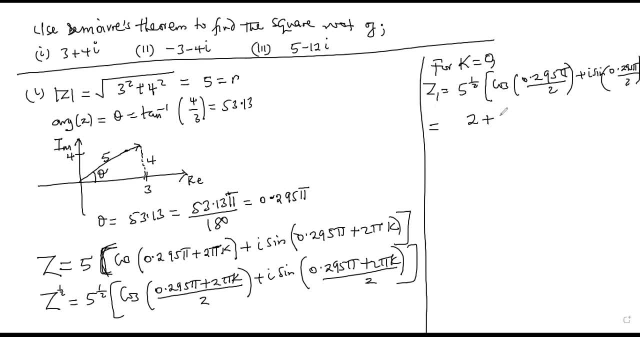 plus i, two plus i, all of it, because this plus i send this times, this reduce to two plus i. then, for k is one when k is equal to one, which means that we have our z2, so it will be five power half into course. now it means that where k is, 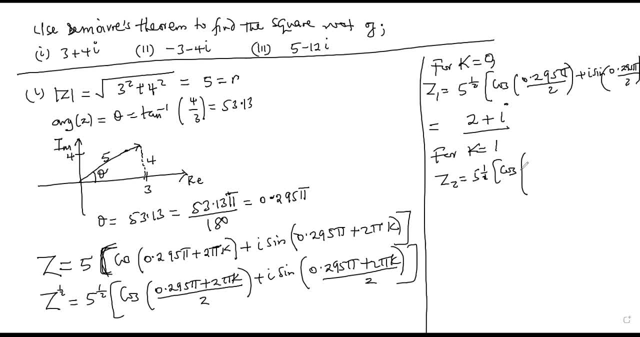 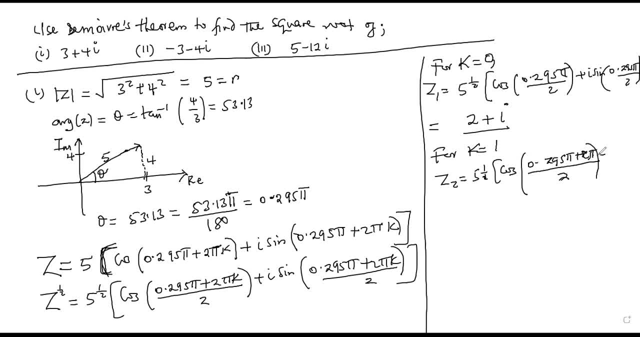 so we shall add two pi out plus k is one, so we shall add two pi out of plus i plus- i remember the whole of this is- is inside of five point power half. so i is inside of five point power half. so i sine 0.295 pi plus 2 pi out of 2.. 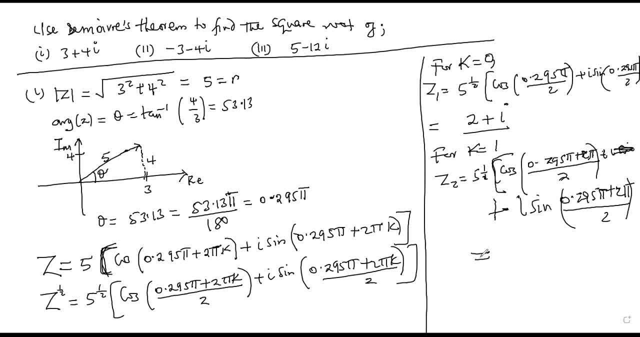 So when you simplify that you're going to get negative 2 minus, i So implying that the square root of 3 plus 4i is equal to plus or minus. 2 plus, i Mean that you're going to have positive of this, then it's negative. 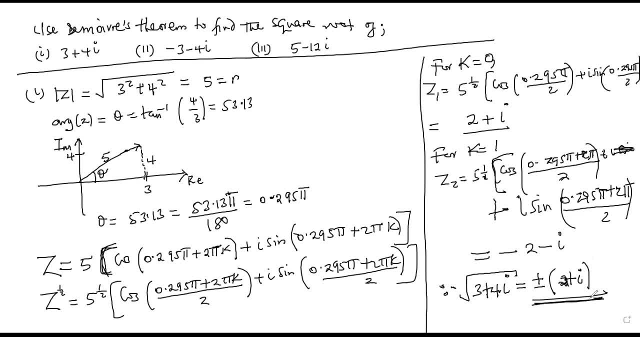 So that is how we get the square root We are going to. We should do very many examples here so that we trigger your understanding. So let's do number two And you see. So that's part two, Where you had three. 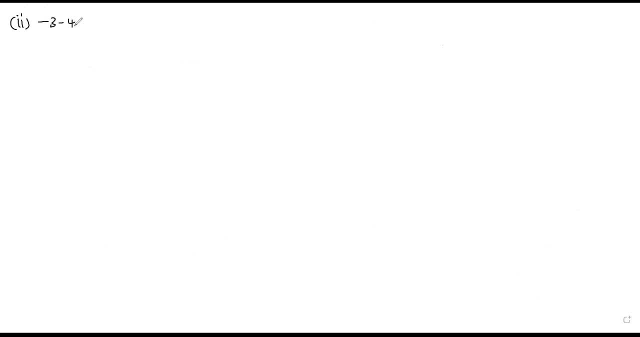 It was negative 3 minus 4i. Okay, So the magnitude of Z, which is equal to R, will be going to the square root of negative 3 squared, That's negative 4 squared. So it's going to be still fine. 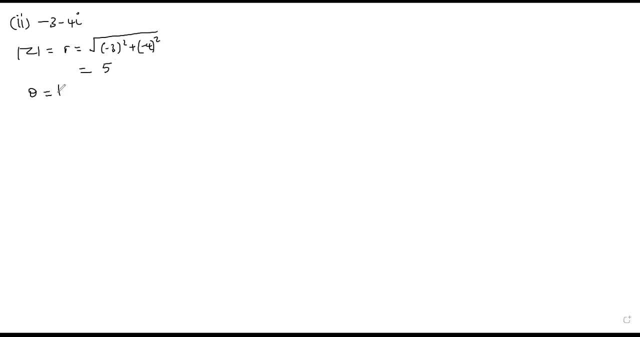 And theta will be according to tan: inverse of negative 4 out of negative 3.. That is the argument, which is 53.1 Therese T, but out of the sketch you can really see in which quad land it lies. 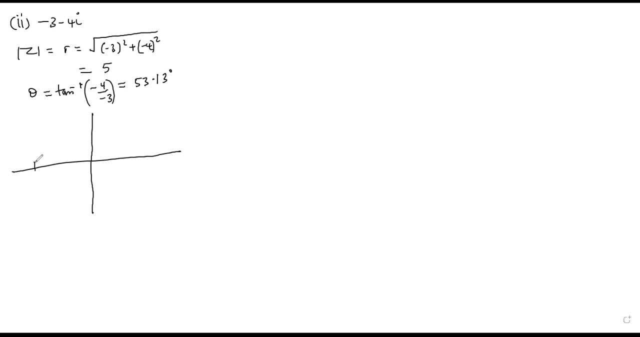 We have negative 3 and we have negative 4.. So when you plot them, you find yourself here. So this is the imaginary and this is the real part. Okay, So we have this meaning. if this is 53.1 theory, what would be the angle from the positive x-axis? 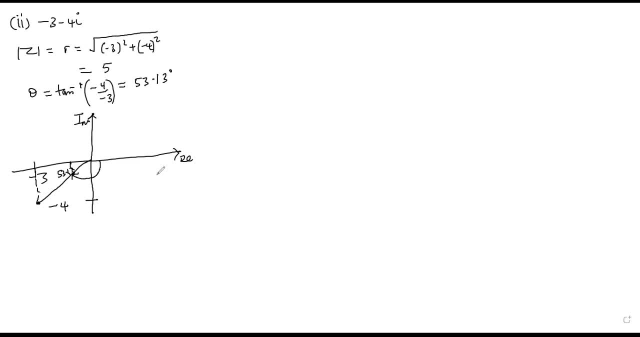 The angle from the positive x-axis, theta will be in the third quad land, which will be negative 127.. We come from the positive x-axis. When you convert this one to radians, it will be negative 127. So we have this. 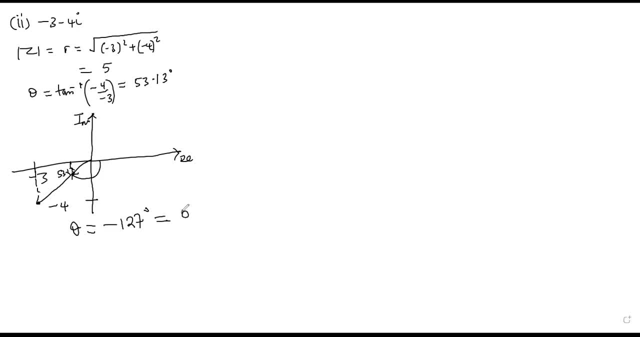 Negative 127 pi out of 180.. That gives negative 0.7. Pi. Now this one would mean that Z power I have Be equating it to five R, That is, R for a half Into Cause theta. 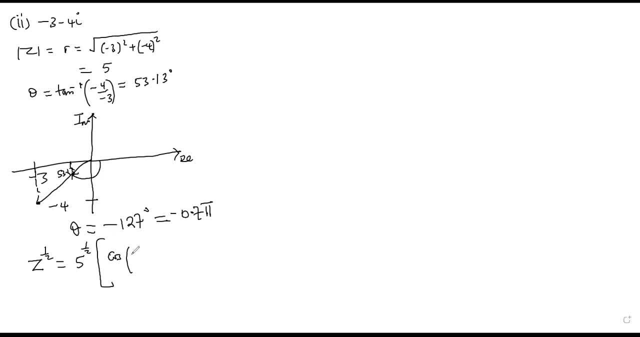 Which will be Course Negative Zero point: Seven Pi Plus two pi k. Out of two, Two is always the value of n that you have been Plus I sign Negative zero point seven pi Plus two pi k. 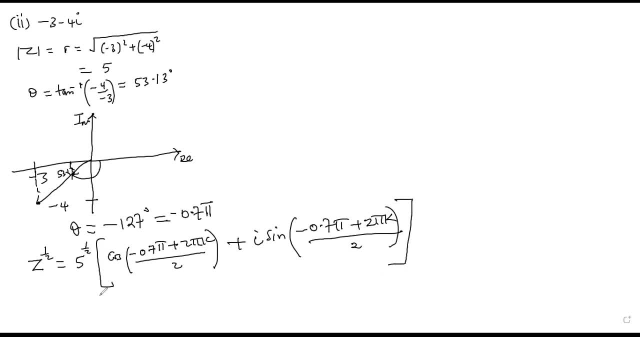 Out of two. So for K is equals to zero. We shall get z one As five power half Into Five power half into Now. the whole of this is zero. So we have cause Negative zero point seven pi But two plus I sign. 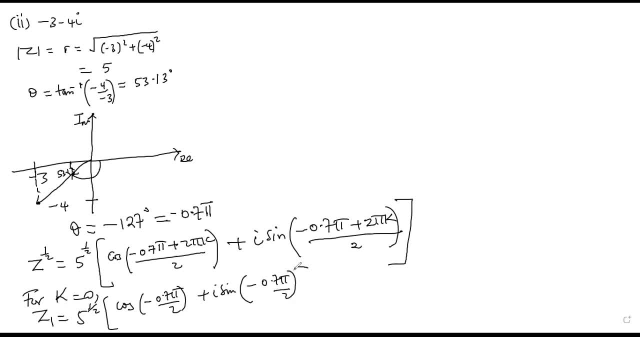 Negative zero point seven pi Over two. Computing is computed: is multiplied by five power half. We're going to get One One In this Part, Minus Two Pi Minus two I. So That is the first value. 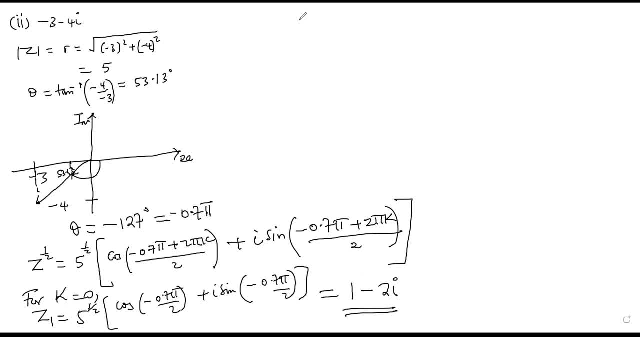 Then, Since they need the square root, It means n is two. So For k Is equal to one, We shall get Our z two. It will be five. power half Is equal to one, We shall get Our z two. 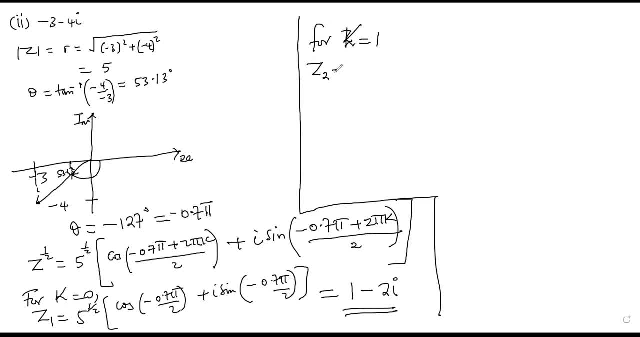 It will be five power half Is equal to one, We shall get Our z two. It will be five power Half. Into Course Negative zero point seven. Pi Plus Two, pi Over two Plus I sign. 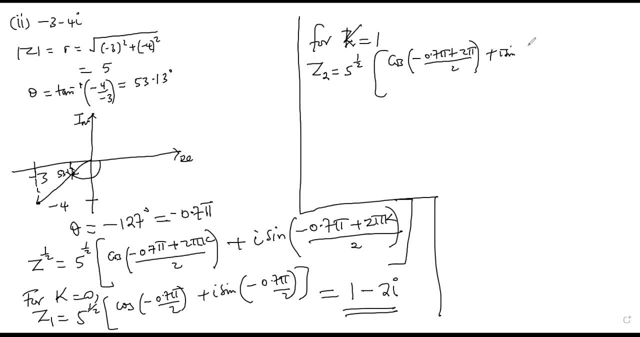 Negative zero point seven. Pi Plus Two pi Over two. So This is Of Course. You have First Added This And This, So This Is One. So It Will. 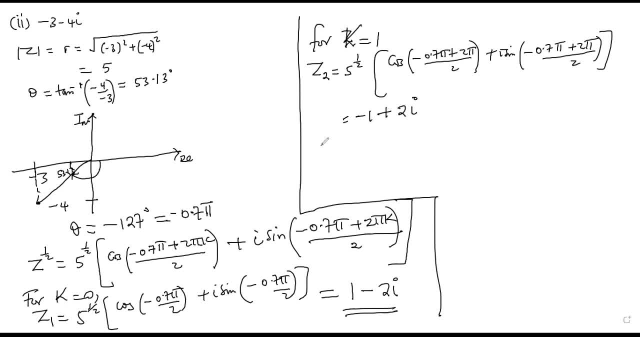 Come To Negative one Plus Two I, Implying That Our Square Root Of Negative Three Minus Four I Is Equal To Plus Or Minus One. 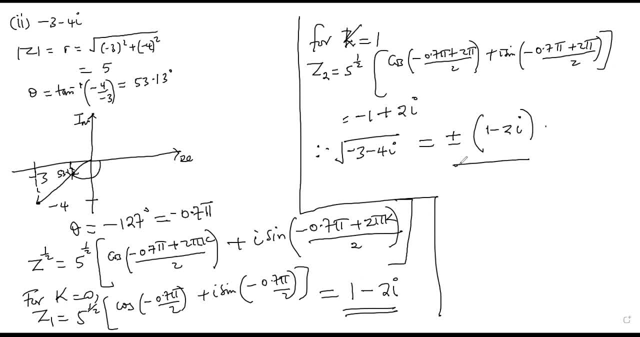 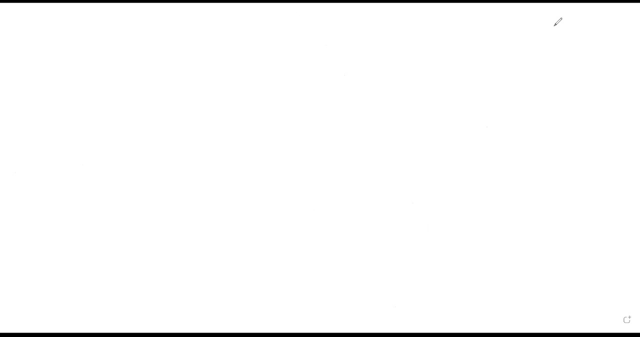 Minus Two Negative Of That. As Simple As That. So Try Part Three, But I'm Still Continuing With Many More Examples. Hmm, Evaluate Negative Sixteen. 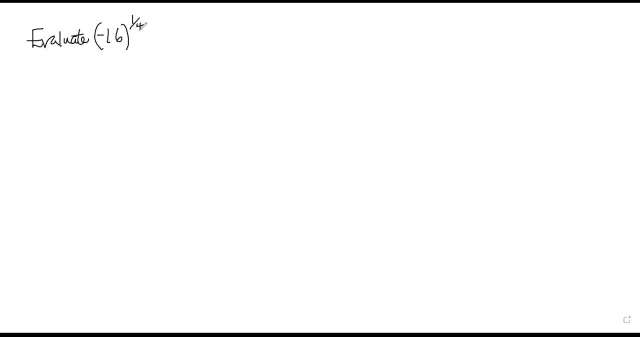 Power Quarter. Or Someone Can Say, Find The Fourth Root Of Negative Sixteen. So That Question Can Be Examined In Those Two Ways, But Still 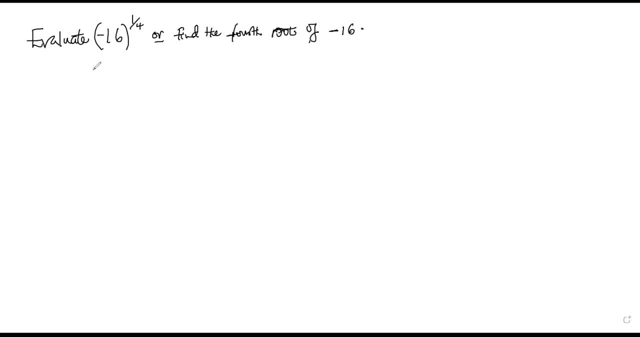 Very, Very, Very Easy. Now, Looking At This To Fourth Root Of Sixteen, What Do We Do? We Shall Let, Let, Let, Let, Let Let. 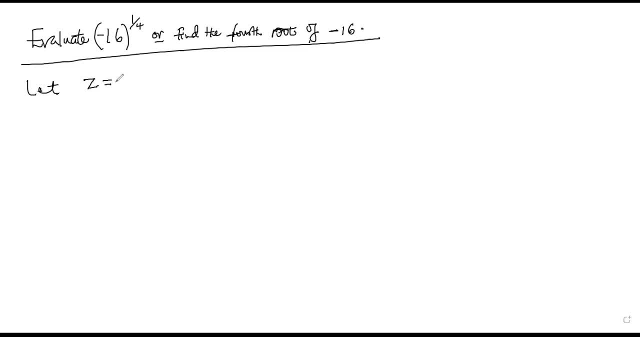 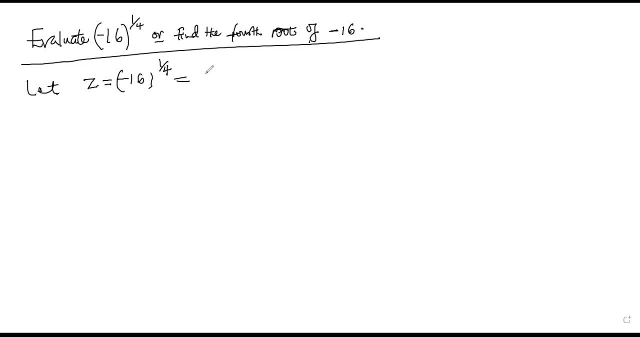 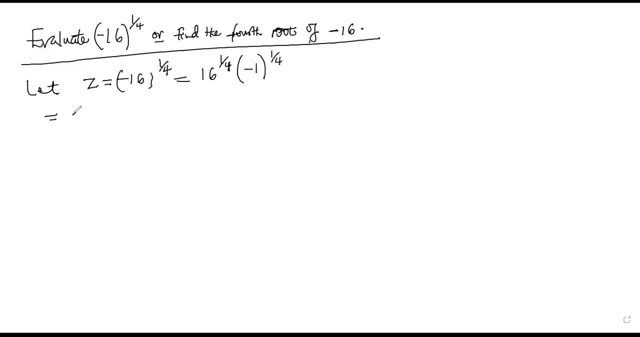 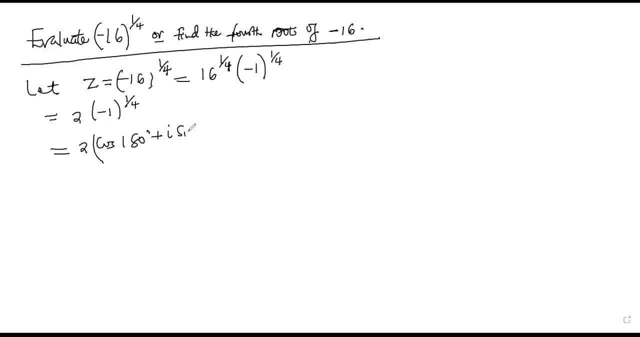 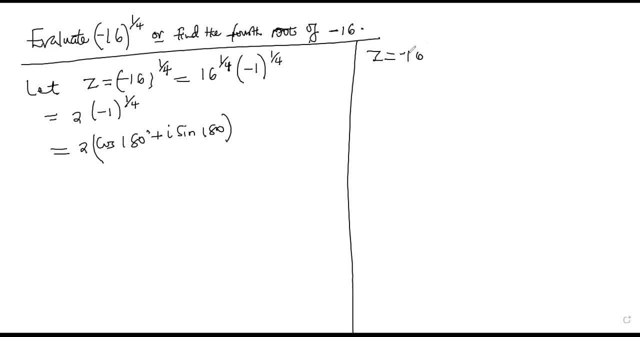 since i let zed to be 16 per quarter, then uh, it would mean that this is the same as negative 16 plus zero i we don't have the imaginary part, but power a quarter. so look for, uh, if i let, maybe my p, if i let p to be. 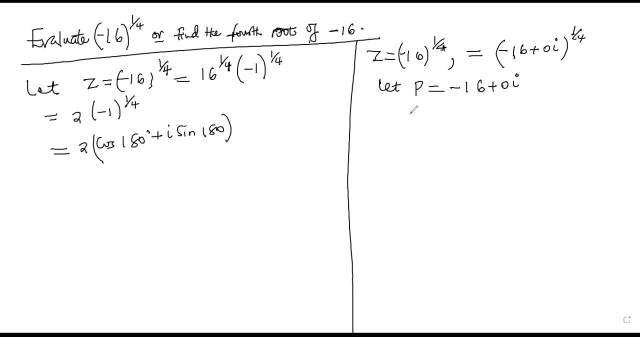 negative 16 plus zero, i can get magnitude of p. magnitude of p is the square root of negative 16 squared, which will keep 16. then argument argument of p will be equaling to uh turn inverse of y component, that is, zero over negative 16.. 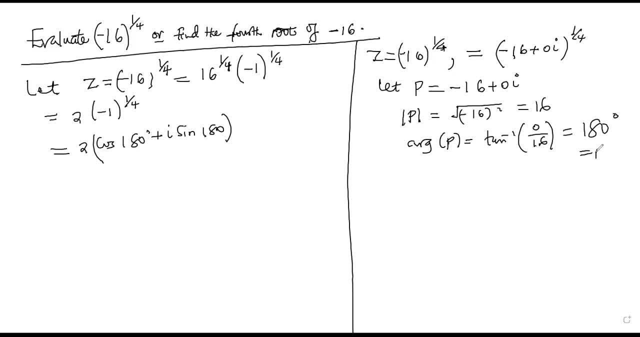 so this is giving 180 degrees, which is pi. all right, but when we are writing we just say that uh zed. uh zed is equals to p power a quarter, because i i relate this one to be my p, so it is p power a quarter which is equals to uh 16 power a quarter. that is r power quarter into cos 180 plus i sin 180. 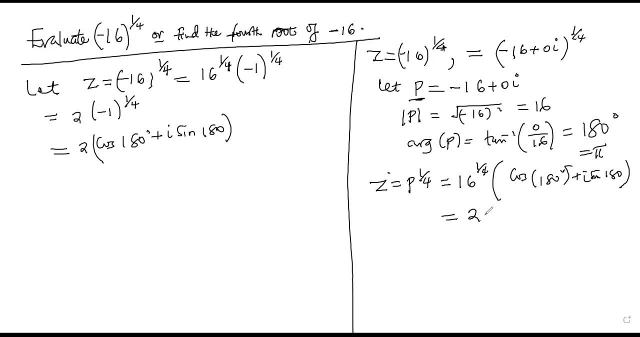 but 16 power quarter is 2, then cos 180, all right, plus i sin 180. so that is where i am now. but remember, i need the fourth root, so i need to go to as far as uh when. if i have this, so it will be. um, once i get this, i need to go to a power piece, and then what you are going to do is you are going to do slope as you get this is it is going to look like this and i can get that two and I'm going to. to a two. and now, if a square root of Cadden, assume that my square root is going to be that we're going to get that two here. so if you're raised to, if you raise the corner, which is about 60, and the gate, which is a square root of where we have it, values. Она subcompathically: 0. that's right. so this is the same as two werk. so that's a power, power, power a quarter, and that's the same as two. în this negative one gives this, but then power a quarter. all right, so by how we can divide things into two, leave r and we could. 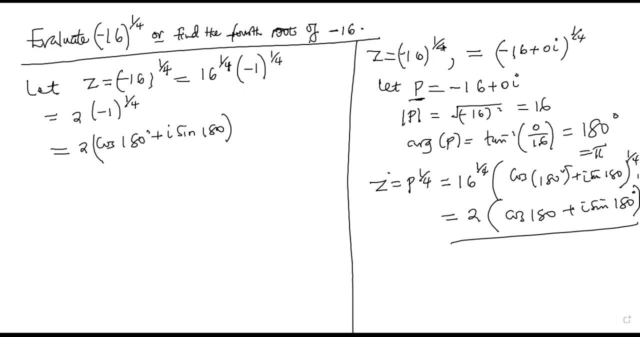 so if r is the same as one, here we divide it into one and click the power a also even here. power quarter, power quarter. So I'm going to have a 2. This negative 1 gives this, but then power a quarter. 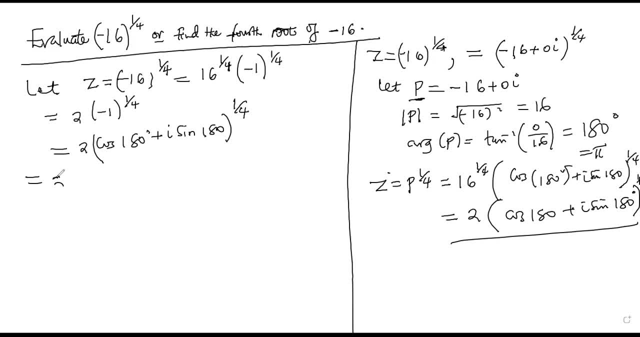 So this is the same as 2.. This is the same as 2 into. of course, 180 is pi. So we'll say pi plus 2, pi k. Now the value of n would be 4,. all right, Plus i sine pi, plus 2, pi k over 4.. 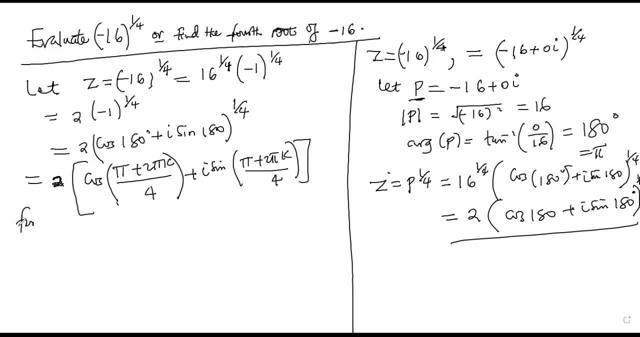 Now we start substituting. 4k is equal to 0.. 4k is equal to 0.. I'll get my z1 as 2.. Of course this is 0. So it will be cos 45 degrees plus i sine 45 degrees. 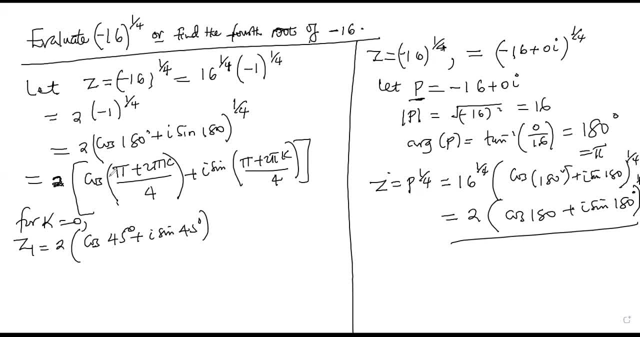 Why Pi over 4 is 180 over 4, which is 45. Cos 45,, then i sine 45. When you compute this, this is going to give you 2.. This is root 2 over 2 times 2.. 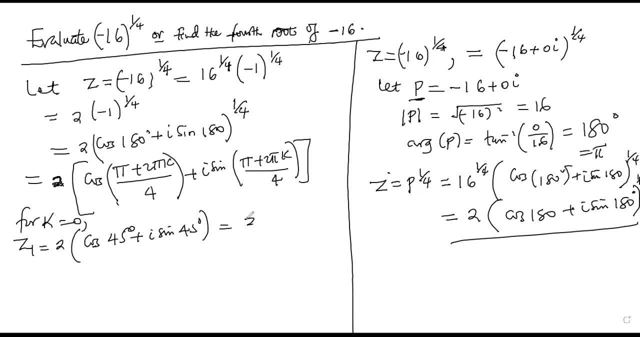 So root 2 over 2.. This is this will be 2.. This is root 2 over 2 times 2.. So this is going to be 2 into root, 2 over 2, plus i root 2 over 2.. 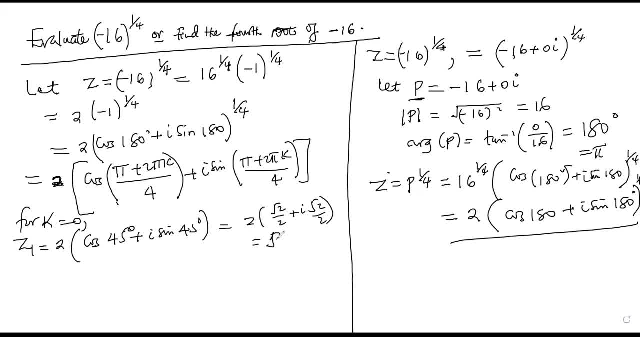 This one is going to cancel, So you have root 2 plus i root 2 as your z1.. Then for k is equal to 1, you'll get z2.. z2 will be 2, into where let's take pi as 180. 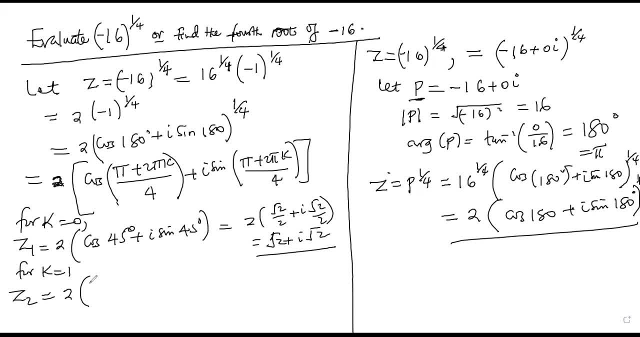 Now k is 1.. Then we divide by 4. So it will be cos 135 plus i sine 145 degrees. So this is going to give you negative root 2 plus i root 2.. Okay, It is still 135 here. 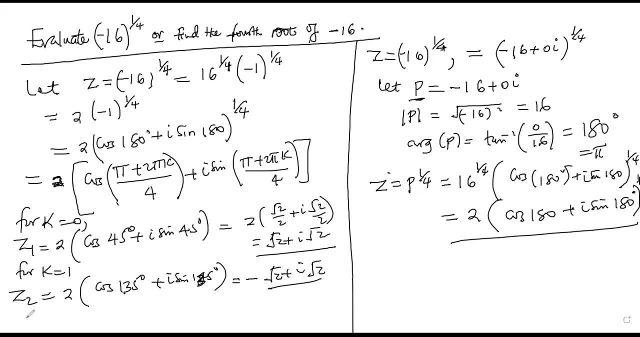 Yeah, So you get this one. So then, for k is 2, we shall get z3. And z3 will be equaling to 2.. Of course, whatever is pi, put 180 and then divide by 4.. So, and whatever that is k, put a 2.. 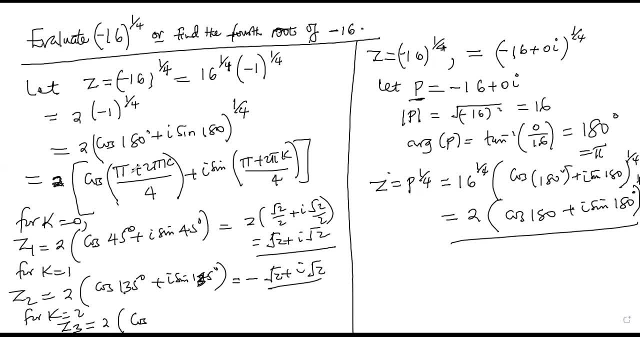 So this will be 4 pi plus pi, That is 5 pi over 4.. Or you can leave everything in pi. Still it is. It is okay. Okay, So cos 225.. Even if you live in pi, no problem. 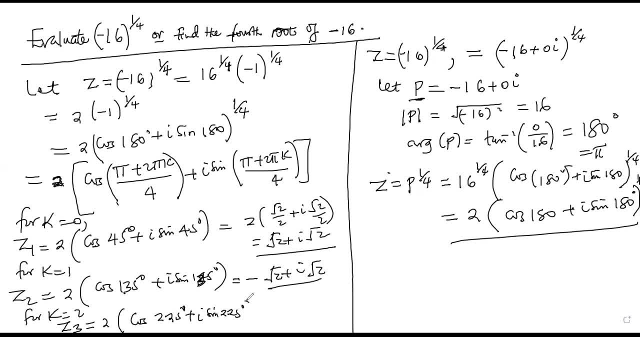 Then plus i sine 225 degrees. So this is going to give you negative root 2 minus i root 2.. Then, finally, for k is 3.. That is when we get z4.. Okay, For k is equals to 3.. 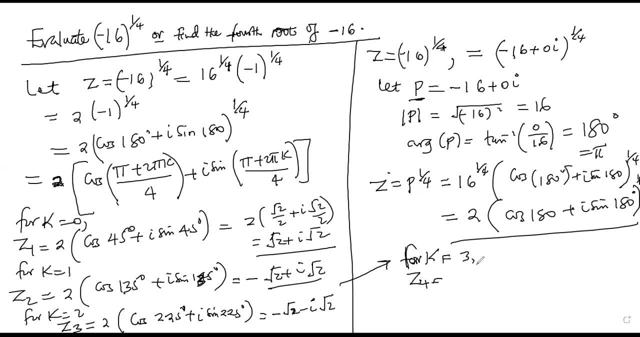 That is when you get your z4.. And it will be 2 into cos. Whatever that is k. now you are going to put 3.. So this is 6 pi plus pi. That is 7 pi over 4.. That is 180 times 7 over 4, which will give 315. 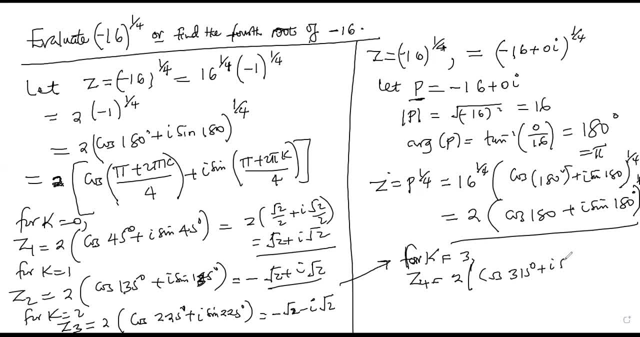 Otherwise I've said you can leave it in pi form. Then plus i Sine, 315 degrees. So it is going to give you root 2, minus i root 2.. So that is my z4. And that is where I am stopping. 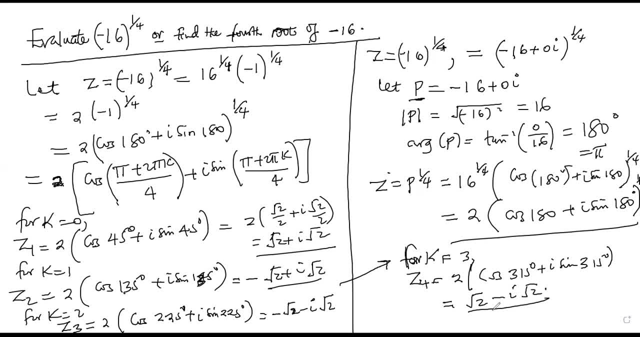 Zeta 4.. After getting z4, we shall compare and say zeta 4.. The fourth root of negative 16 is going to be equal to plus or minus root 2.. On whatever case, we have either positive root 2 or negative root 2.. 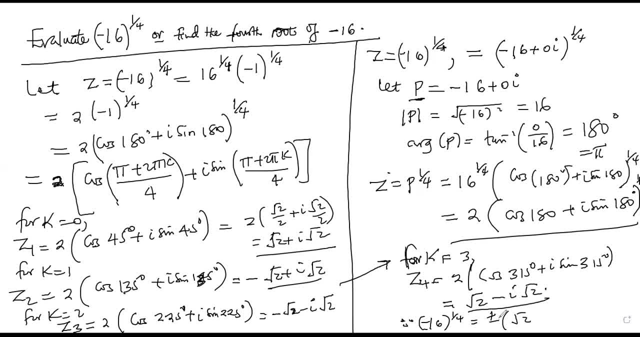 So that's why I'm saying: plus or minus root 2.. Then plus or minus, i root 2.. Why am I putting another plus or minus? Because we either have minus i or positive i. So that is what we have as our fourth root. 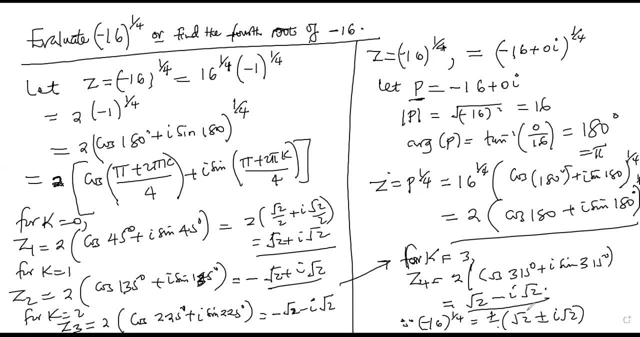 or you can write all of them. you can write all of them. you can write this comma, this comma, that comma, all of them. you can write this, this, this and that, all of them. so let every viewer be. i'm continuing, though, but let every viewer find the chubu root. 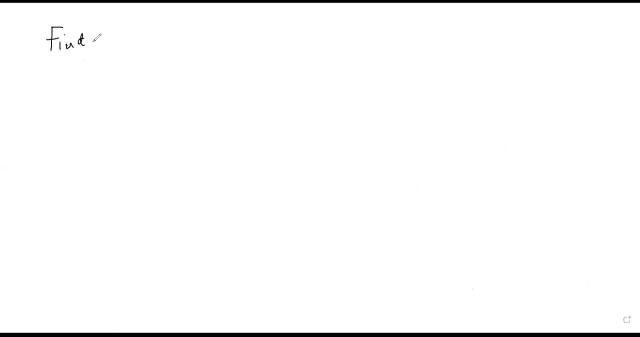 find the chubu root of root. no, no, no, no of 27 i. that is for everyone watching this lesson. okay, i'm going to do more two questions. i'm going to do more two questions, and then i call it a time with the demover's theory. 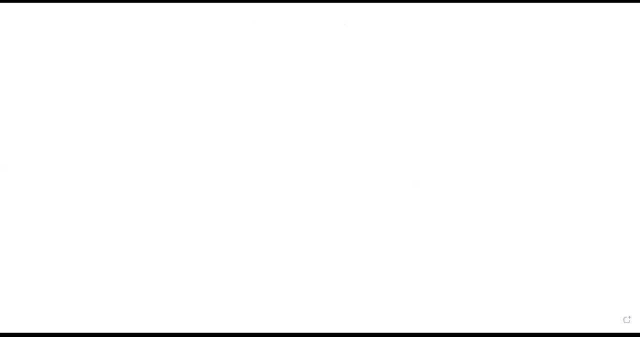 so find, find, find the roots of z power. 4 plus 4 is equal to 0 using demover's theorem. so uh, for this one here you need to be very smart. so for this one here is a expectation of z power 4. this is say, z power 4 over z is the. 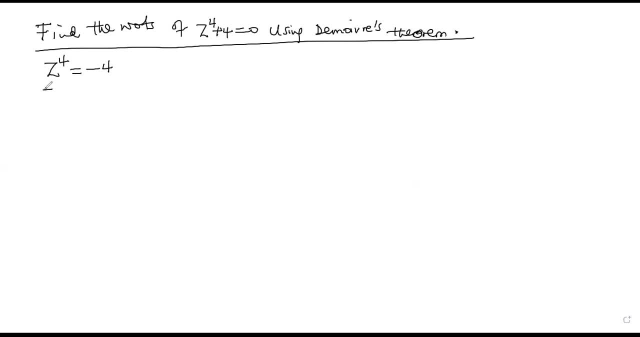 right way of explaining this why z power 4 work in this example? because there's another random fraction. let us said z power 4 is equal to zero. let us say z power 4 is equal to negative, 4, 0i, which can be taken as z power 4 to be equaling to negative, or I can call it 4,. 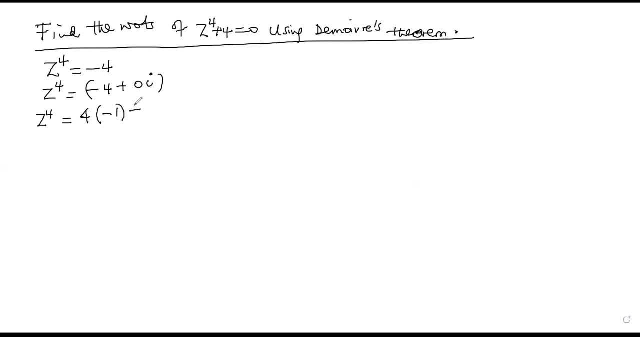 into negative 1, sorry, sorry for this step. I can call. I can say z power 4 is equal to a 4 negative 1 plus 0i. So having this, I can get my argument. my argument of z will be equaling to tan inverse. 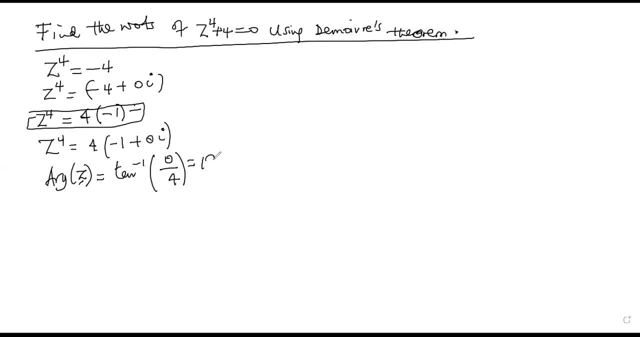 of 0 over 4., Which is 1i. similarly pi right, Then my modulus of z is going to be equal to the square root of negative 4 squared plus 0, which is the same as 4.. Implying that z power 4 is equal to 4.. 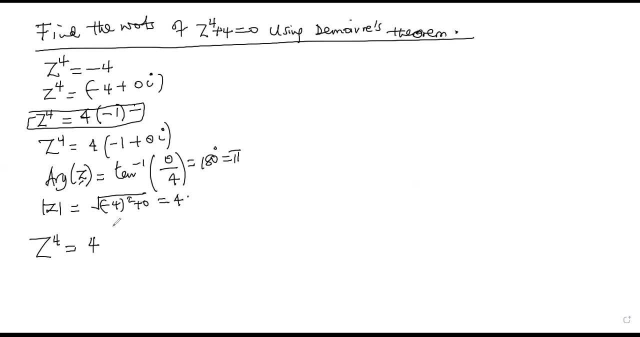 This one in polar form. it is this one in polar form. this complex number in polar form is cos 180.. Okay, It is cos 180 plus 0.. Okay, Okay, This is cos 180 plus i sin 180, right. 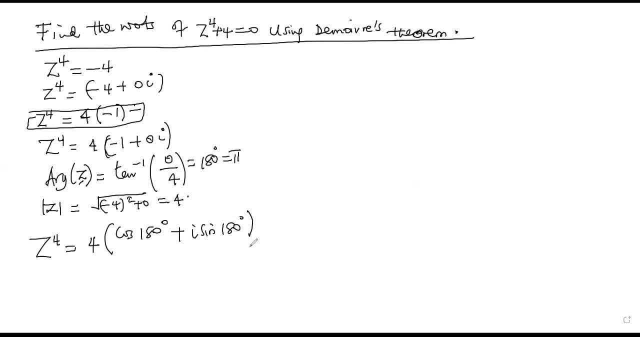 Mm-hmm. So relating to relating to what we have already done. so it means that our z power 4 is equal to 4 into 0. Okay, Okay, Okay. So, relating to cos, this is 180, which is pi plus 2 pi k. 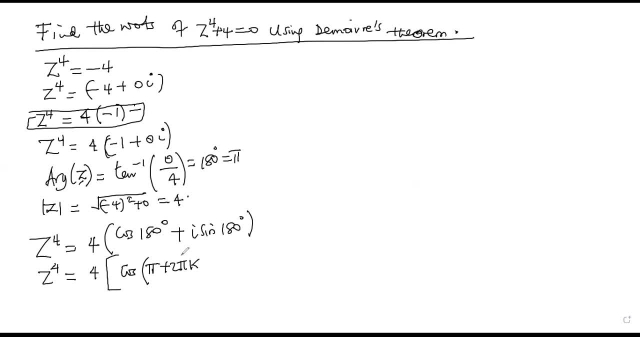 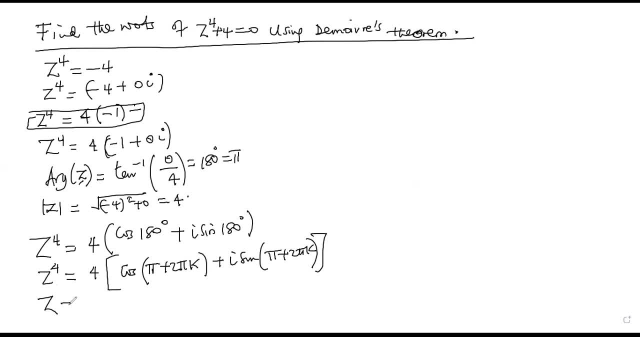 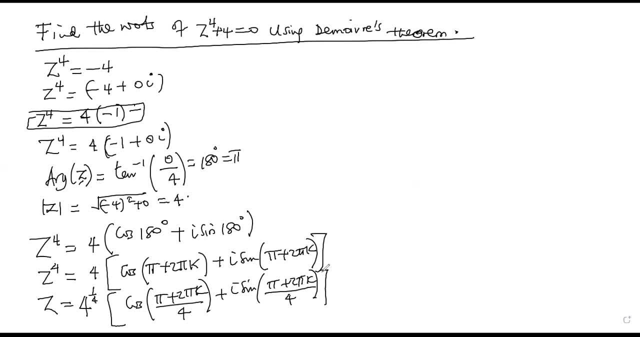 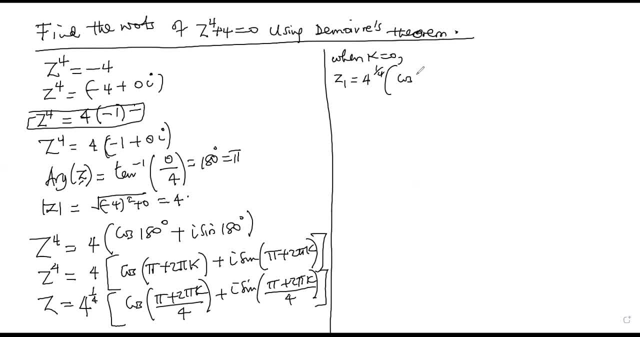 Let me, Let me take a break, Okay, Okay, so we don't have this part. so cos pi over four plus i sine pi over four. so this is the same as we summarize this up: the fourth root of four. the fourth root of four is root two. 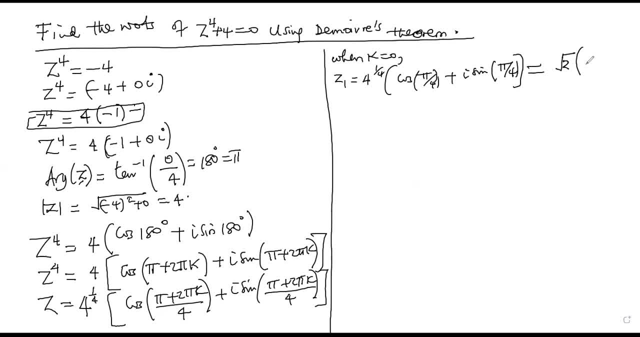 so we shall have it as root two out of. uh, rather into cos, pi over four is one over root two. when you say pi over four, look at 45, then plus i sine that, which is one over root two also. so this one will reduce to one plus i. 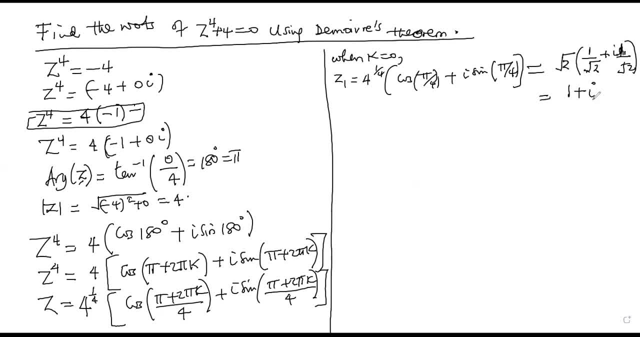 whereby this one and this one will make a one, this one and this one will make one, but we have, i that same. so uh-huh, for k is equals to one, we shall get z2. so z2 would be equaling to four power quarter and two. 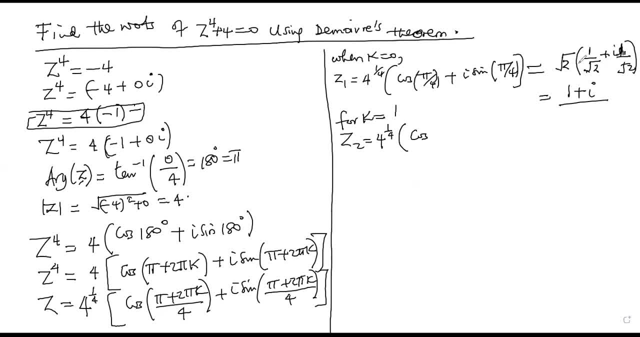 otherwise some students who don't know how to express these ones in sad form. they maintain decimal points, which is okay, of course, pi over four. but when k is one, whatever that is the k, we shall be putting it one. so, uh, now this one becomes two pi, two pi plus pi over four, it becomes three pi over four. 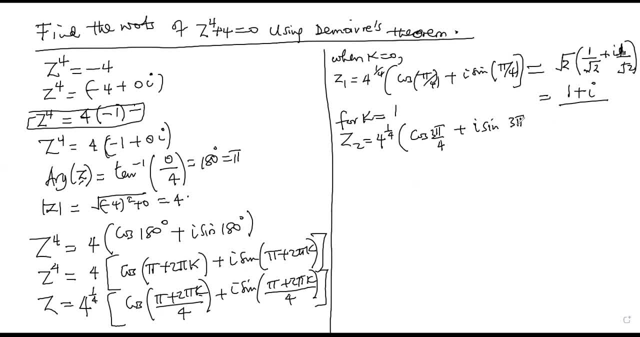 plus i sine three pi over four, plus i sine three pi over four, plus i sine three pi over four. all right, so that's it. so this is root two cos three pi over four is negative. one over root two. sad form members, let's learn how to get these angles in that form. 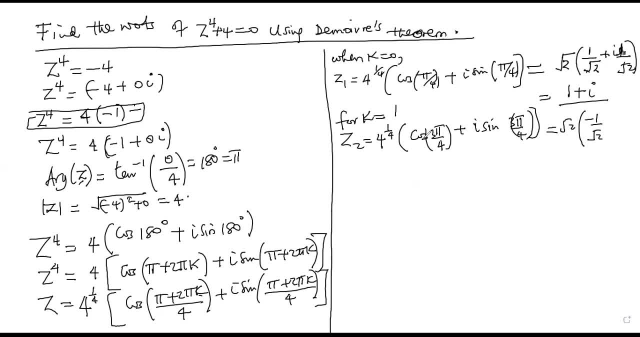 or you maintain: pi take. put your angle, put your calculator in radians and take cos three pi over four. uh, then plus I, 1 over root 2.. So this is going to reduce. You'll get your negative 1 plus I When K is 2,. 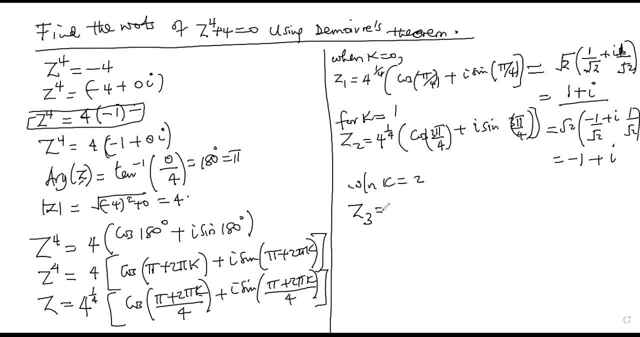 we get Z3.. So Z3 is 4 power quarter into cos. Now this one, we have 4 pi plus pi, That is 5 pi. So we have 5 pi over 4 plus I sine 5 pi over 4.. 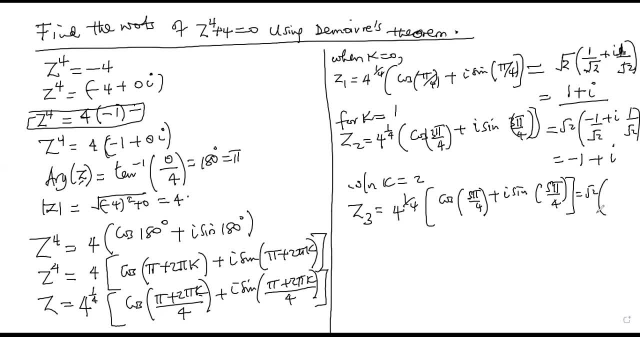 So this is going to be root 2 into. this is negative: 1 over root 2 minus 1 over root 2.. But with the I. So this is going to be negative. This is going to be negative 1 minus I When K is 3. 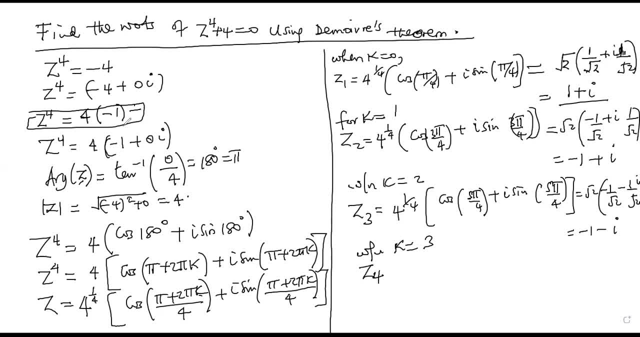 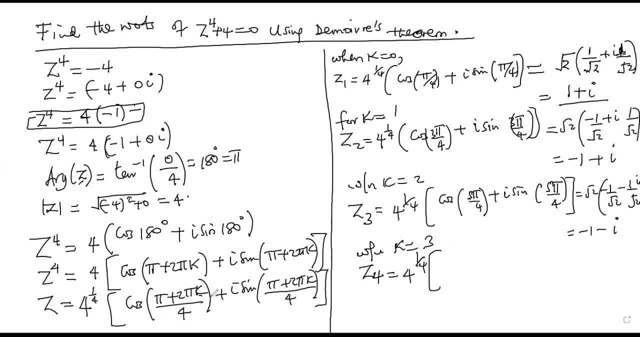 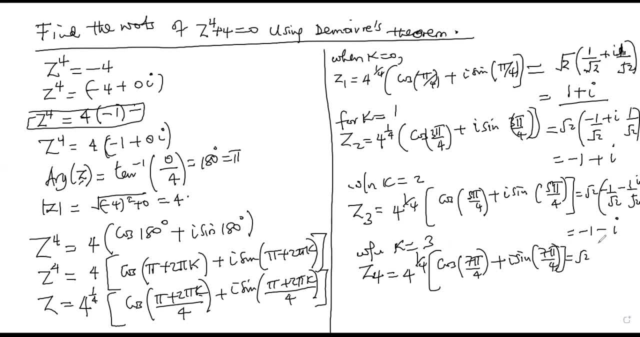 this will be root two into one over root two minus i, one over root two, so it will be one minus i, applying that, therefore, the roots of z power four plus four r. you can list all of them, or you can say this comma, this comma, this comma and this comma, or can summarize them as: because you have one plus. 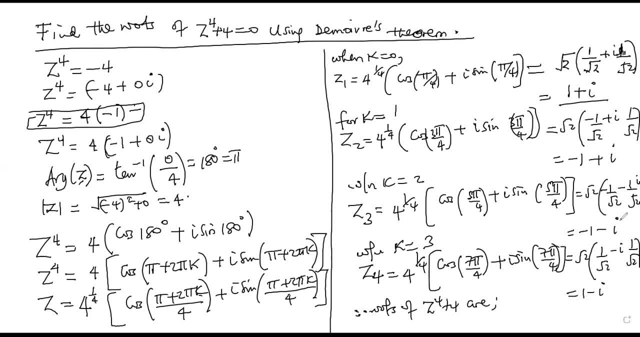 i, and here you have one minus i. you have negative one plus i, you have negative one minus i. so they can be one plus or minus i, because here you have one plus i and here you have negative. or another one easy: here you have negative one, negative one, so it can be negative one. 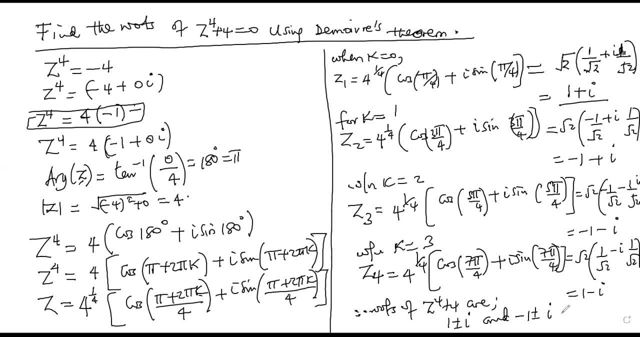 then plus or minus, i. so if you cannot, if you cannot get uh, these, uh angles, rather these values in root form, then you record your decimal places and be accurate. see, you'll be fine when your calculator is in the radians, but this one here requires you to practice to know what is three, pi over four, which angle is that and what. 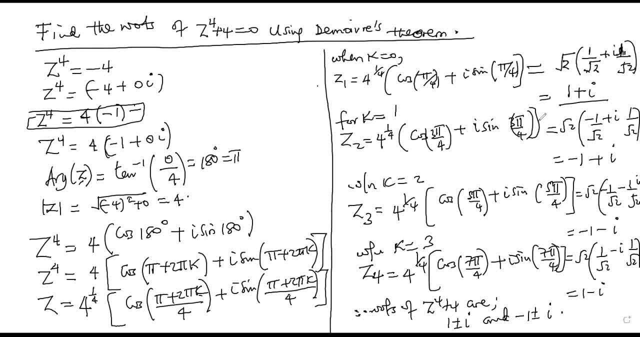 is it when i take that, when i take the other sign, then you can't explain it like aetti. right, there is also the of of that angle which takes you back to trigonometric to see how that trigonometric ratios match with the suds. okay, so let me do my final question. let me do my final question and then 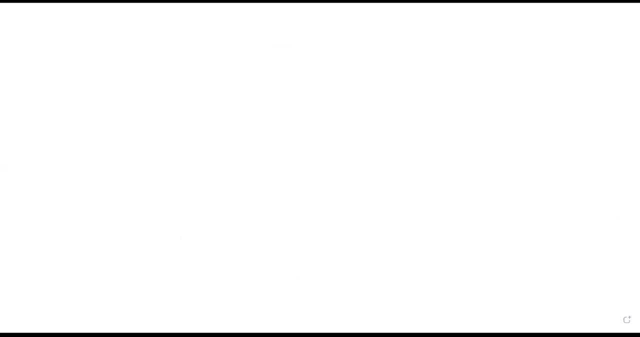 you see? yeah, in case i see any other questions to add on, i'll be adding on. but for this, this, you can go toEerma. just add oneoker to the 여�yetime, which we take it to been TiEermaай guess, okay, nice, yes. 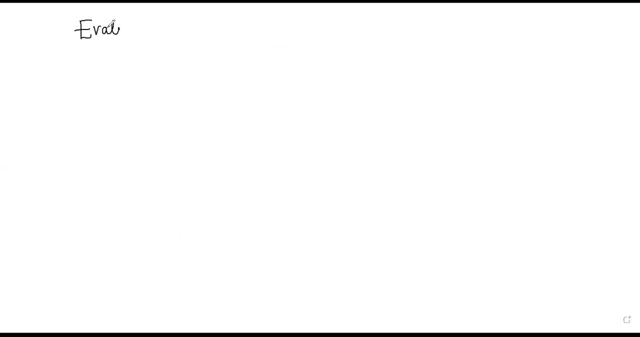 will be sum of enough. evaluate: one plus root, three, two thirds. okay, that is what we are having. evaluate that. so let's see how we do evaluate this. so solution: one plus root, three or two out of three. let me say that this is the same as one plus. 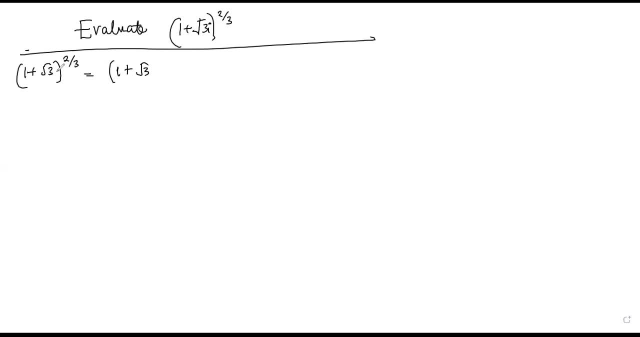 actually was root three. i yeah, we have root three, i. so the question is one plus root three, i, so three, i right, so i can say squared. then power a third, so that i bring in the element of root, because when it is two thirds it becomes somehow tricky for us. okay. 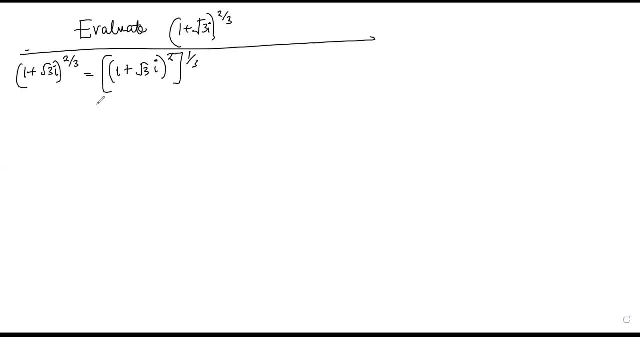 uh, so this is the same as one plus root three. i times one plus root three. right, then i've had this is this is what brings in power two thirds, because when you add the power one, power one becomes two squared. this is squared, then power third, implying that: 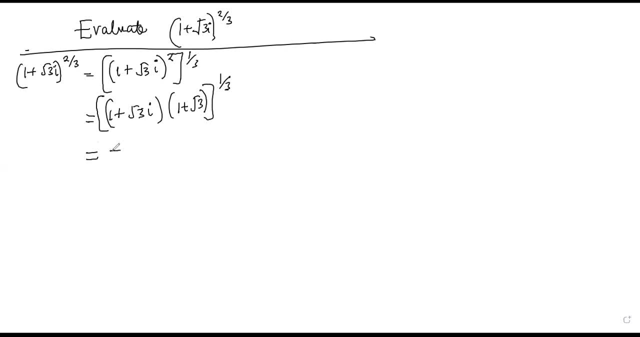 when you simplify this, it's going to be negative: two right plus two root three. i then to the power a third. how does it come about? right plus two root three. i then to the power a third. how does it come about? remember, as i did all this so that i meant i have that, that the, a third, the, that the root. okay. 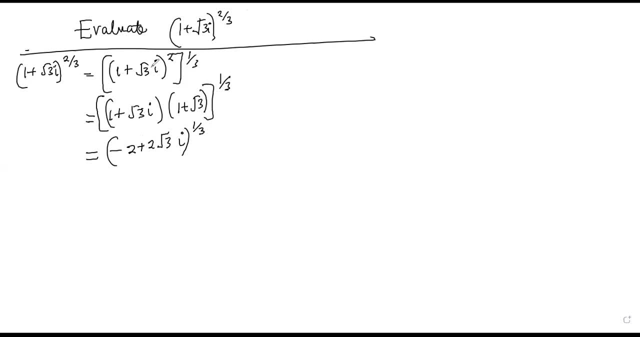 but when it is two thirds it is hard for you to express. so, having brought two inside, it's a square. that's why i spread these two. so i have one times one, which is one, then one times root three, that is root three. uh, one times this, root three i, and then root three. 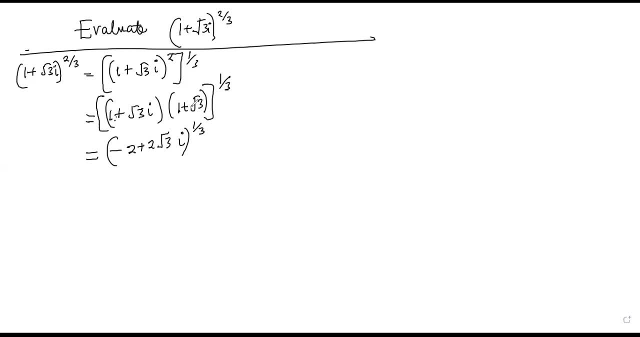 i root three, i times root three, we shall have three. okay, it comes to three, i right, okay, so one plus root three. i times one plus root three. i- oh, there is another. i here. so the expansion: one times one, you get one. this one is coming from. 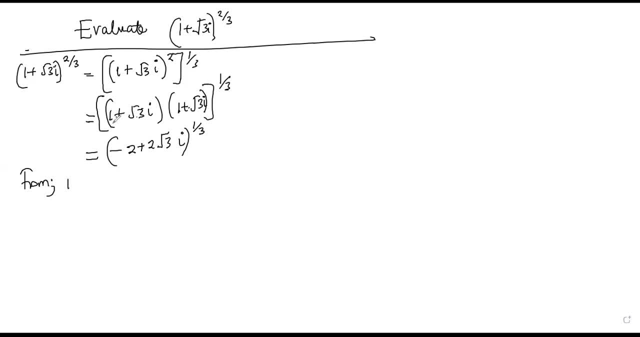 one times one, which is one plus root three i plus another root three i. then because of how it was keeping puisque k of this negative to be minus three, because i times i is negative one, but root three times three is three. so negative three. one minus three, that is negative two, root three i plus root three. 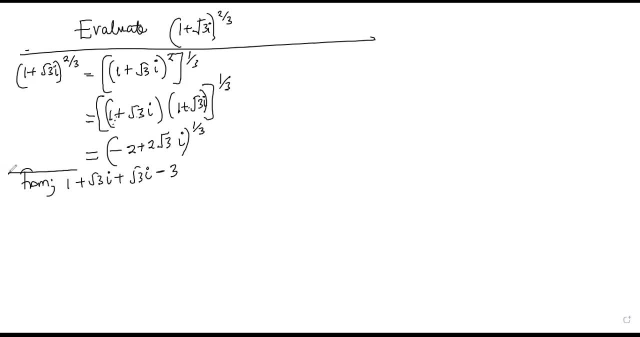 i, that is, two root three i. so, uh, having obtained this, it means that i will let, if i let my z to be equal to negative two plus two root three, i. okay, uh, so i can get my magnitude of z, which is going to be equal to the square root of negative two squared plus two root three. 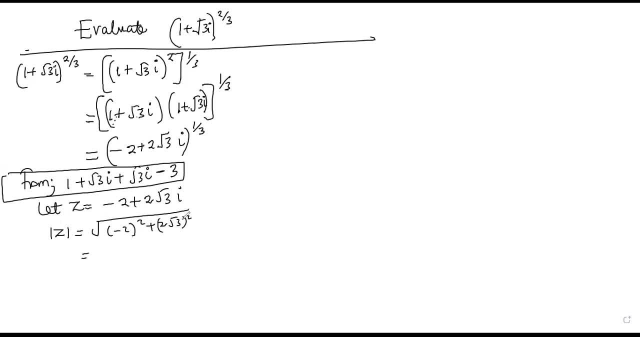 everything squared, so this is a four, then a four that's for 16, so the whole result will bring it to a four. okay, so this is four gz4 plus two squared gz4 times three, 12 and a root which gives a four. so after having written this, we can go ahead to look for the argument of z. argument of z is the tan. 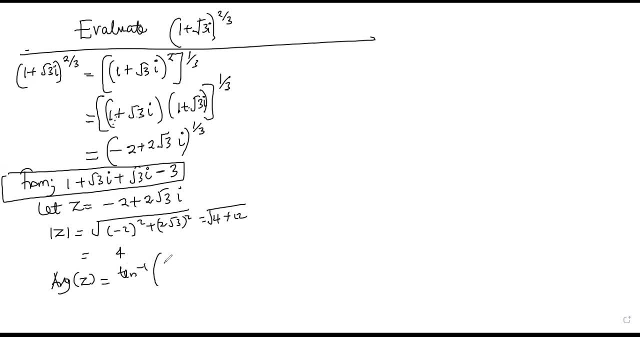 inverse of two root three, that is the, the imaginary part, over negative two. so this is going to give you, of course, this: the tan inverse of c negative root 3 equals a 2, with a 2 will cancel, which will give you negative 16. uh, but, but you. 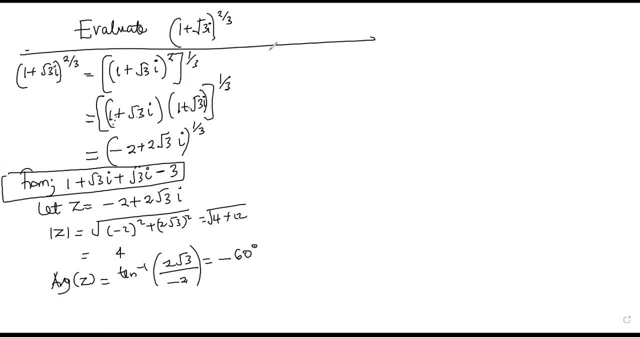 need to sketch so that you know in which quadrant are we lying, in which quadrant are we lying? so if we do sketch that we have our real and we have our imaginary. our real is negative 2, while our imaginary is 2 root 3. so, uh, we are here. 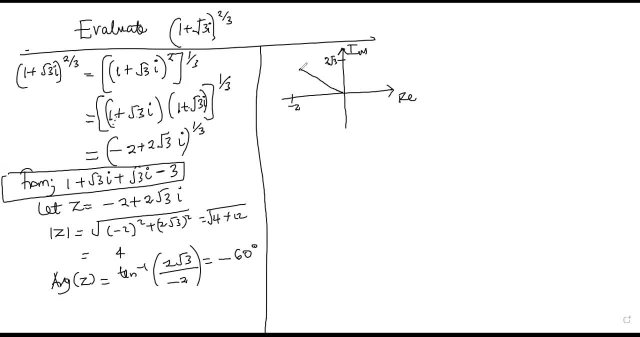 in other words: uh, we are in the second quadrant, okay. so this way, in the second quadrant we are looking for this angle from the positive x axis. so if we get our theta so as 60, we are looking for this angle here. so it will be uh. 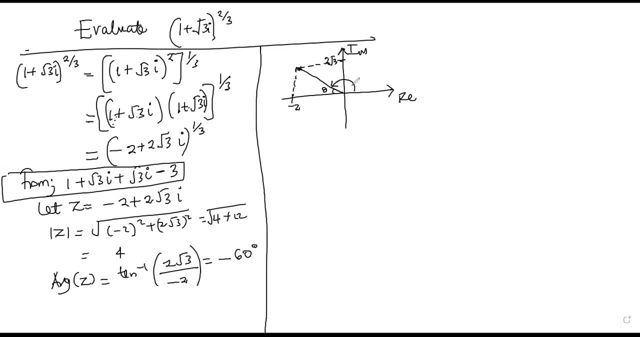 180 minus 60, which will be 120. so our angle will be 120. so it means that this is equivalent to 120 degrees, but 120 degrees the same as 2 pi over 3. why do i get 2 pi over 3? get 120 pi. you divide by 180, you'll get. 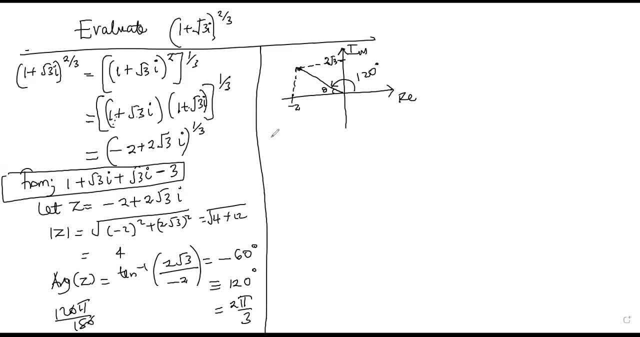 two-thirds pi. so, after having gotten this, it means that our z. you'll get two-thirds pi. so, after having gotten this, it means that our z. so, after having gotten this, it means that our z. now, if i'm to write it in polar form, it's going to be a four. 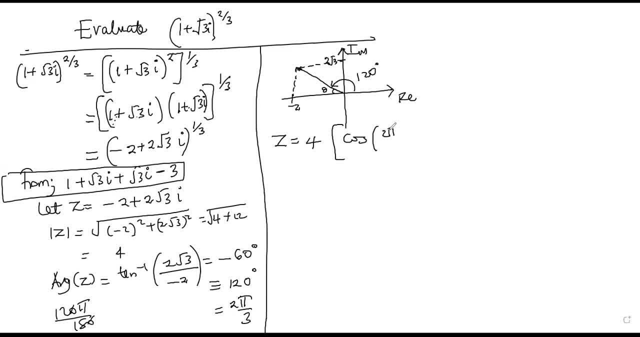 then of course theta, which is two pi over three plus two pi k. then plus, i sine two pi over three plus two pi k. okay, so, uh, it means that z power. third, because we are looking at a tube root. now we reduced it up to the tube root so that there about that will be equaling to here you can get the rcm and then 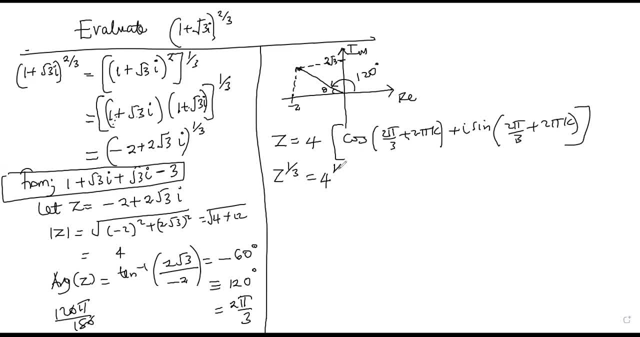 you move a three down, so it is going to be four thirds, four power. third, of course, uh, it will be two pi plus six pi k y, six pi k. rcm is a three. so, uh, it will be over nine. why? because, after getting this rcm here, it 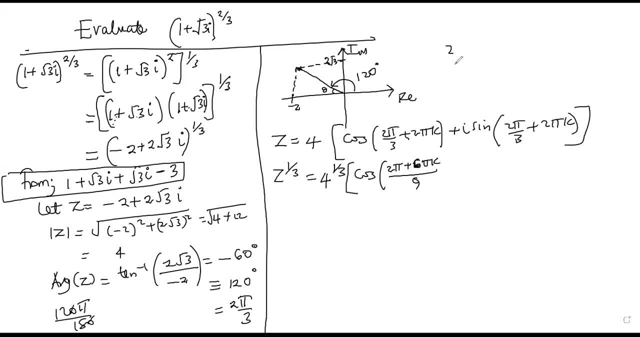 becomes the whole thing. before bringing that two, before bringing a three inside, it is two pi plus six pi k out of three, but then you have to bring the power down, so it will find this three. it makes it nine. okay, plus i sine two pi plus six pi k out of nine. then now we start. 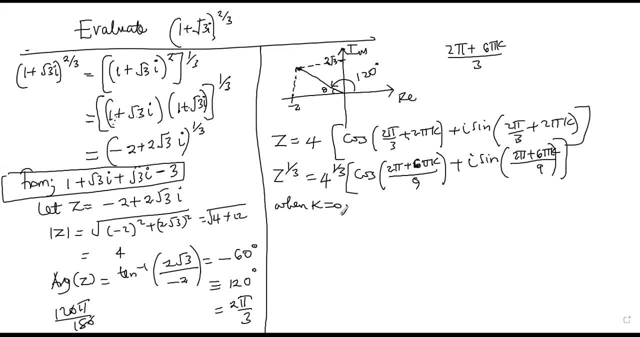 uh, when k is zero, when k is zero, we shall get z one which will be four power. third, into course, two pi over nine, plus i sine two pi over nine. so, uh, this one will get you now, like this one. let me get you my answers in decimals. 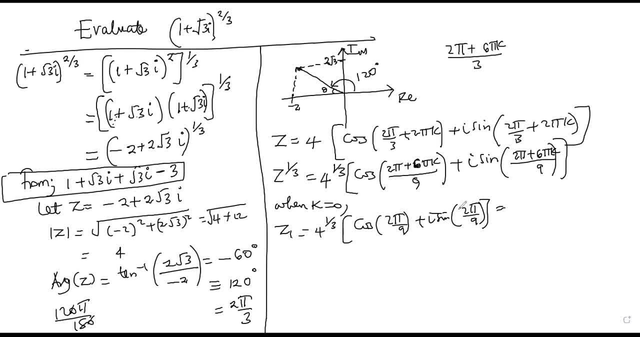 so i get four power. third, I'll put my triangle cos theta and then later in, sine theta. so it is going to be one point two, one six zero plus i, or plus one point two, one six zero, i. uh, when k is one, we get z squared. 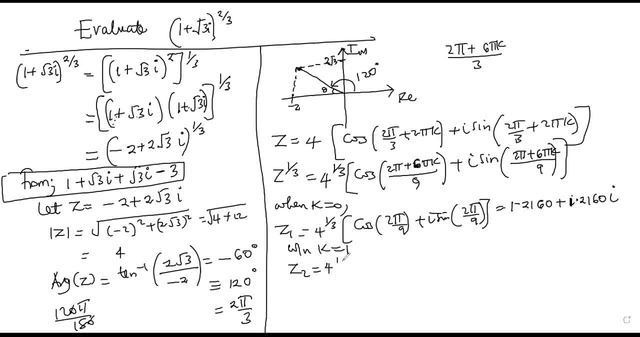 two, so it will be four power third into cos now, wherever k is put: one so it will be eight pi over nine. so eight pi over nine plus i sine eight pi over nine, so it will give you negative when you check the cosine of this and then you multiply four power three to give you negative 1.4917 plus. 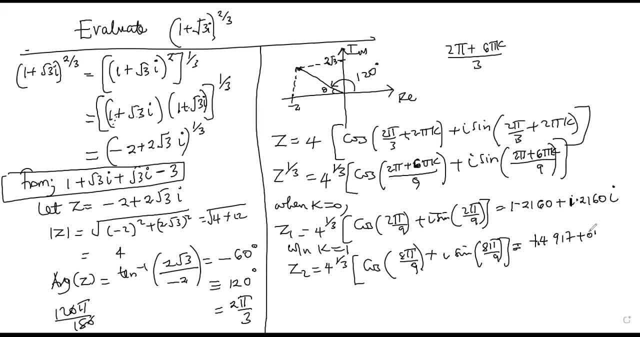 0.5429i. then you go to when k is two. when k is two, that is when we get the third root. all right, the two root before that, four power, third, of course. now when k is two, substitute it will be 12 plus two, that is 14 pi out of nine, 14 pi out of nine. 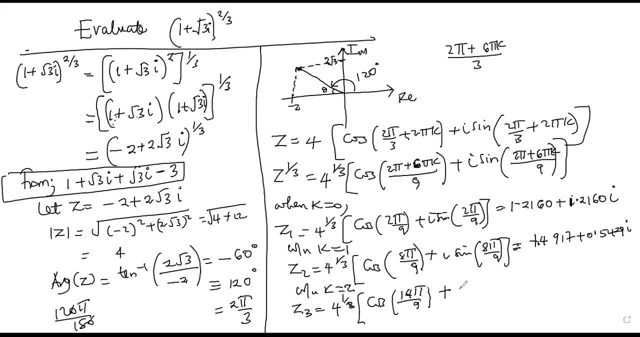 plus i sine 14 pi, 14 pi, 14 pi out of nine. so this is going to be equal to the real part- would be 0.2756, 0.2756. this would be a negative 1.5633i. so we've got an z3. therefore one plus root three. i. 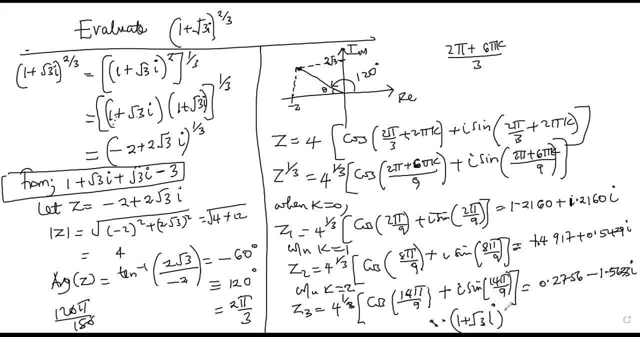 to the power two out of three, to the power one plus one plus one plus two. i r, j r m b. you will write this comma, you write that coma. that is how the answer supposed to be, interestingly, which gives you some numbers to do, but through your analysis, here is what it is to do. 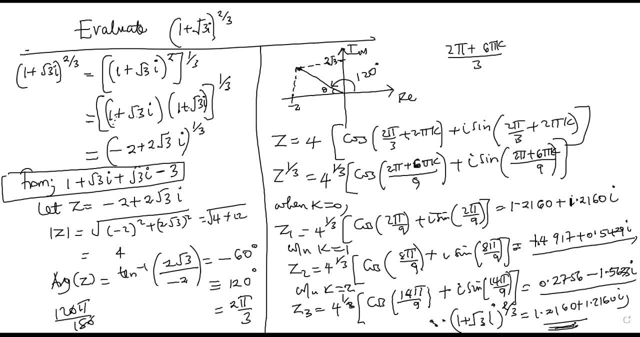 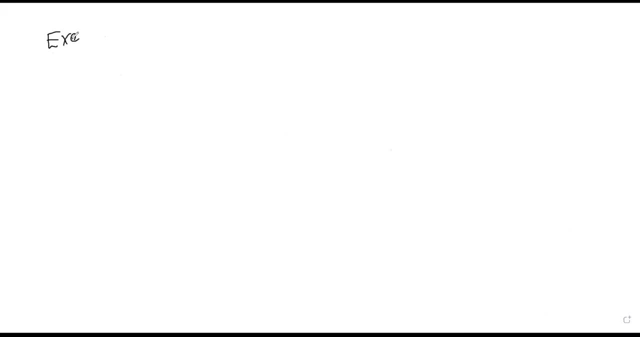 your comments on my youtube channel. i can get try your problems so that i pull you from there. okay, exercise solos z power. four plus one is equals to zero. two solo z cubed plus 27 is equals to zero. of course you strictly use the mobile theorem for your 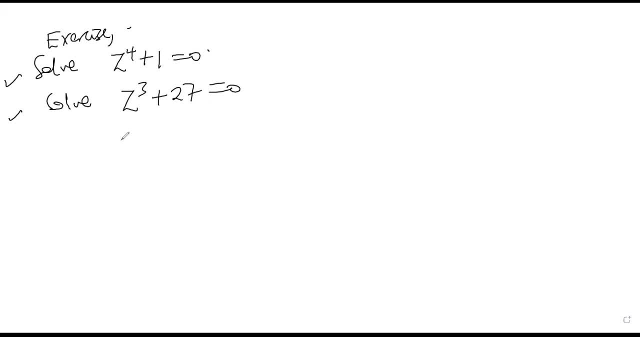 practice so that, uh, you can get it very well, okay, otherwise, the other method is that can get to the answer. but since we are looking at this, let's try to get to the answer. to use a removal steering, then, um you, there are very many numbers that can be done. 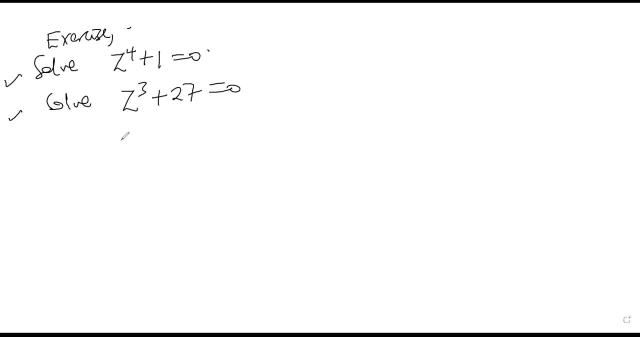 okay, i'll first do this one zambian. so i'm going to do this one zambian. so i'm going to do this one zambian. so i'm going to do this one zambian, luigi. so i'm going to do this one zambian.